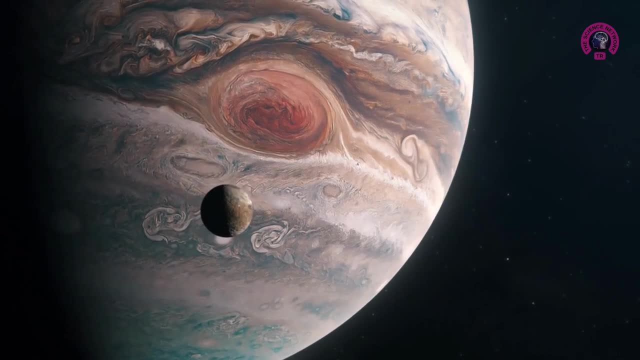 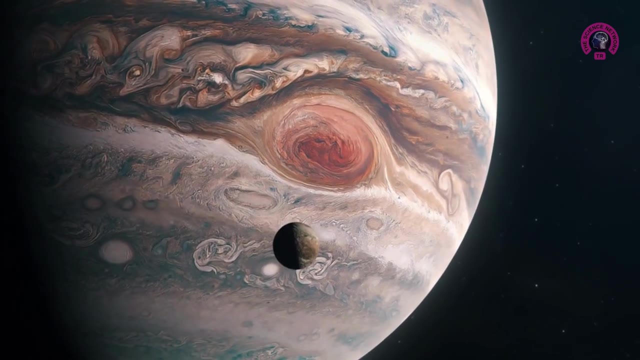 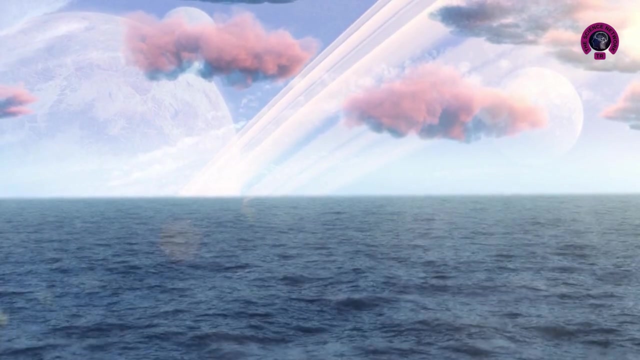 detectors and spectrographs that enable us to peer billions of years into the past. With each new breakthrough we uncover hidden celestial treasures and gain fresh insights into the cosmic tapestry that surrounds us. But astrophysics is more than just a scientific pursuit. It stirs our imagination, ignites our curiosity and evokes a sense of wonder. 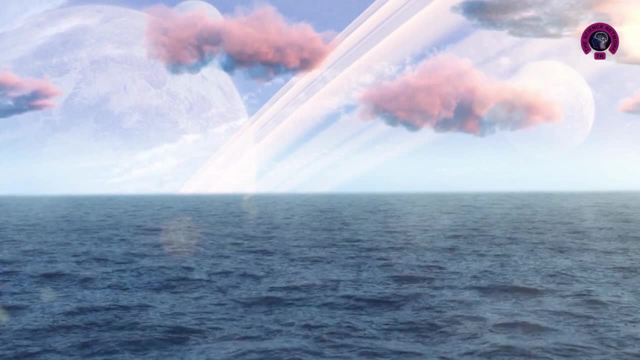 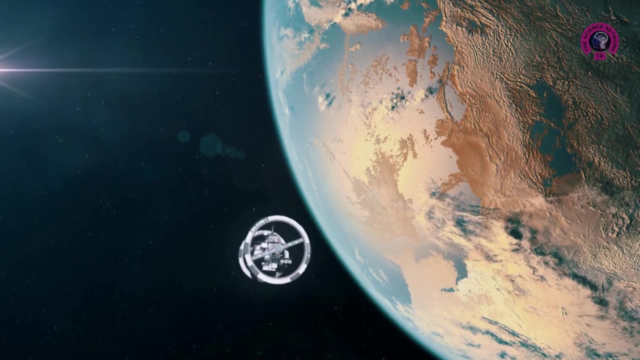 It reminds us of our place in the grand cosmic ballet, where every star, every galaxy and every atom in our bodies is intricately connected. So join us on this exhilarating journey as we delve into the mysteries of the cosmos. Together, we will explore the 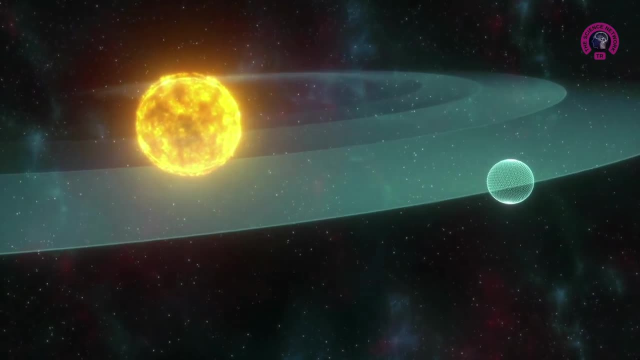 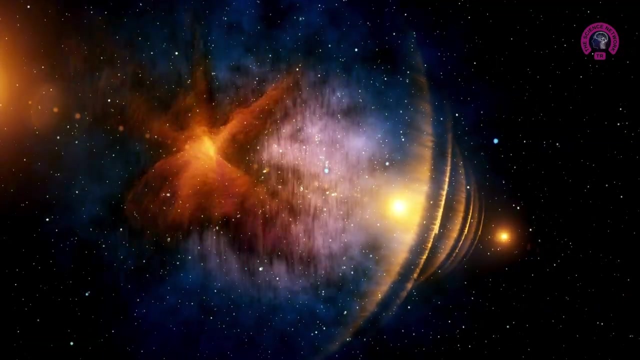 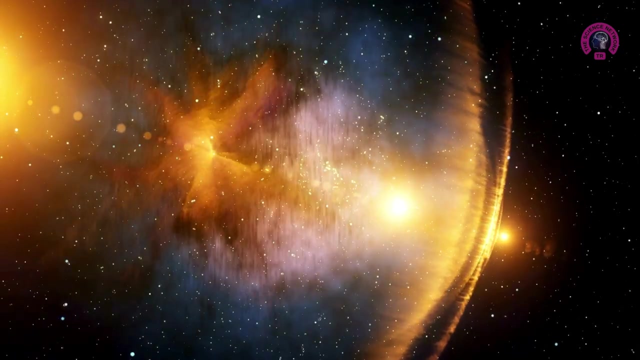 enigmatic worlds of black holes, the dazzling dance of binary star systems, the intricacies of planetary formation and the search for life beyond our pale blue dot. Astrophysics is an adventure that beckons to the curious, the dreamers and the explorers of the 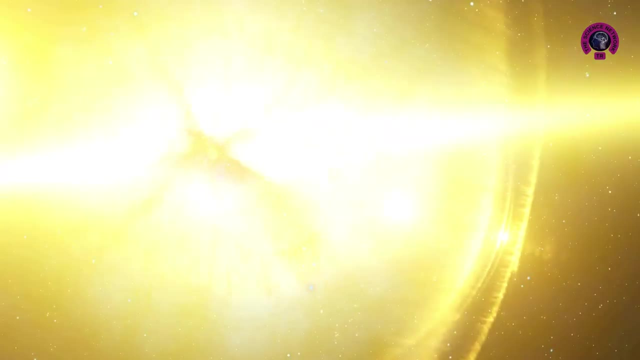 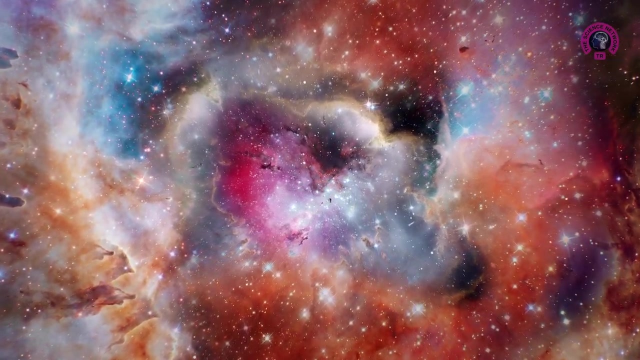 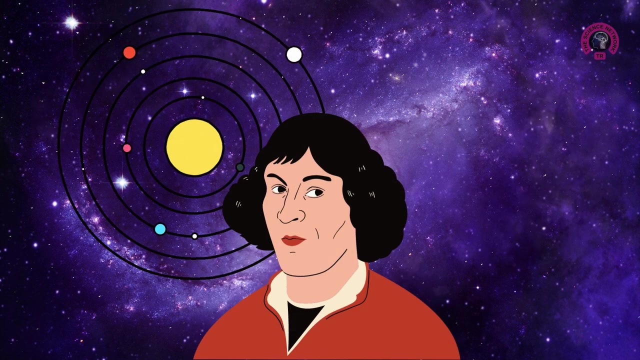 unknown. Get ready to embark on an extraordinary voyage that will stretch the limits of your imagination and forever change the way you perceive the universe. Welcome to a captivating exploration of the historical milestones and brilliant minds that have shaped the field of astrophysics. Throughout the annals of time, courageous thinkers and intrepid observers have gazed at the stars. 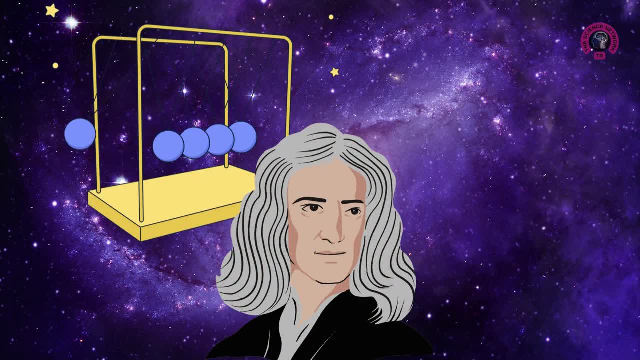 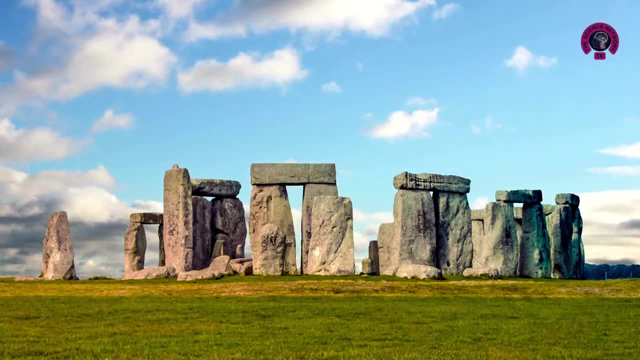 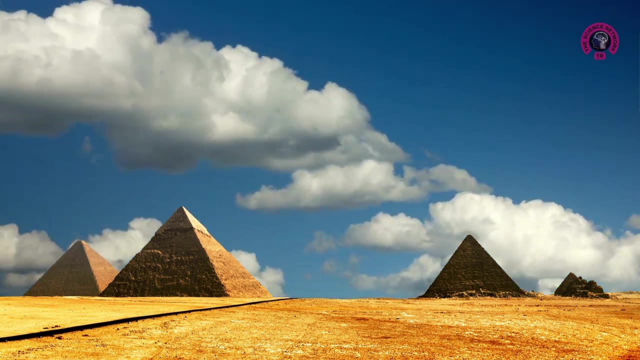 unlocking the secrets of the cosmos and forever altering our understanding of the universe. Our journey begins in the ancient world, where early civilizations, with their celestial observations, laid the groundwork for the birth of astrophysics, From the mysterious stone henge, meticulously aligned with celestial events, to the awe-inspiring pyramids of Egypt. 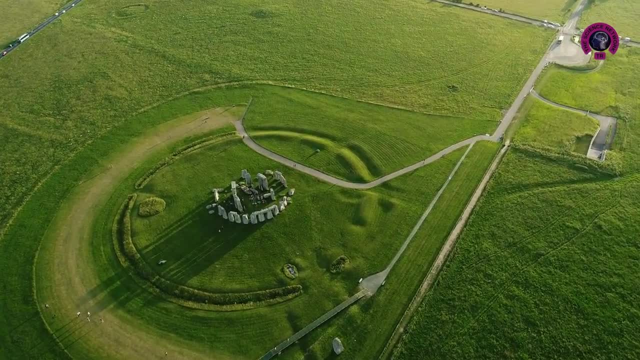 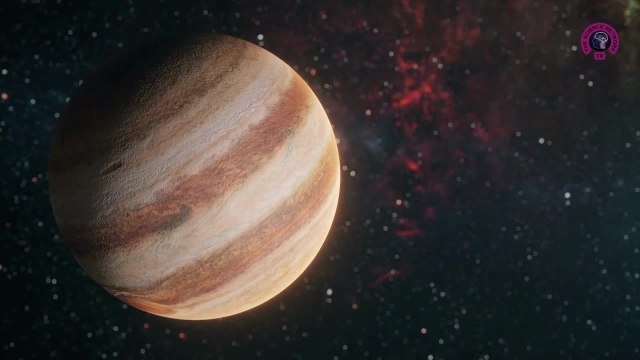 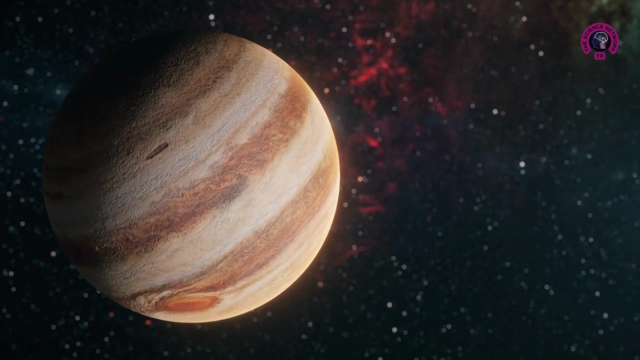 that mirrored the cosmos. our ancestors marveled at the heavens, planting the seeds of curiosity that would blossom into a scientific revolution. Fast forward to the Renaissance, a transformative era when visionaries shattered the prevailing dogmas and ushered in a new era of understanding. 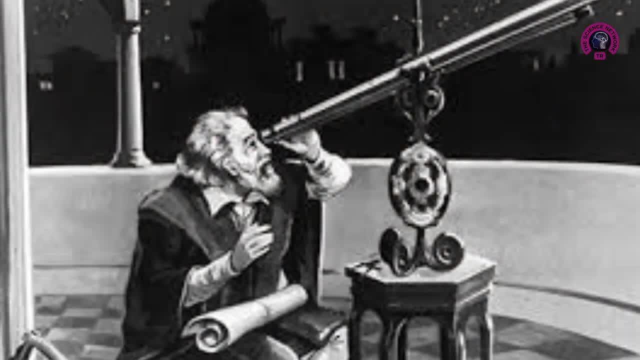 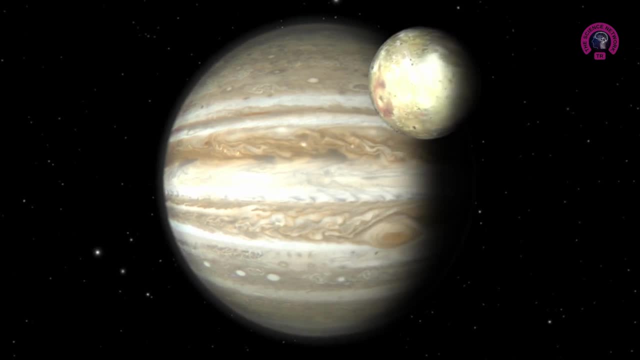 Galileo Galilei, with his groundbreaking use of the telescope, turned his gaze skyward, revealing the craters on the moon, the moons of Jupiter and the enigmatic phases of Venus, Through his audacity and unwavering commitment to truth. 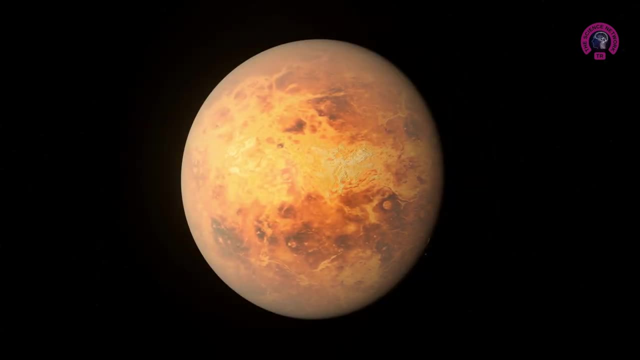 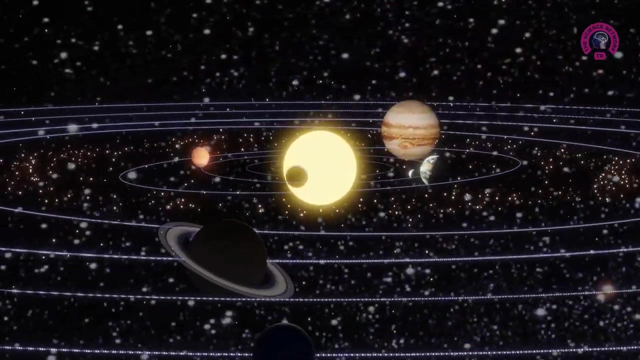 he sparked a scientific revolution that challenged the status quo and paved the way for future discoveries. In this voyage through time, we encounter the monumental contributions of Nicolaus Copernicus, whose heliocentric model courageously dethroned Earth from its presumed 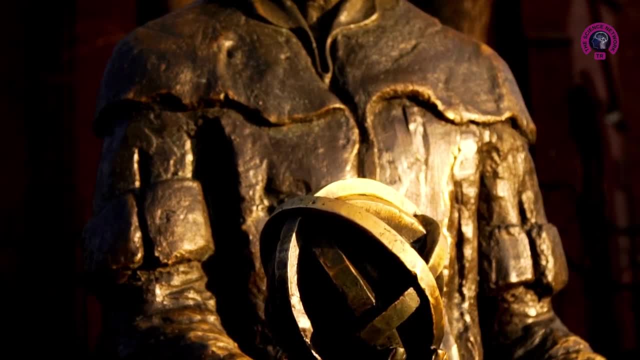 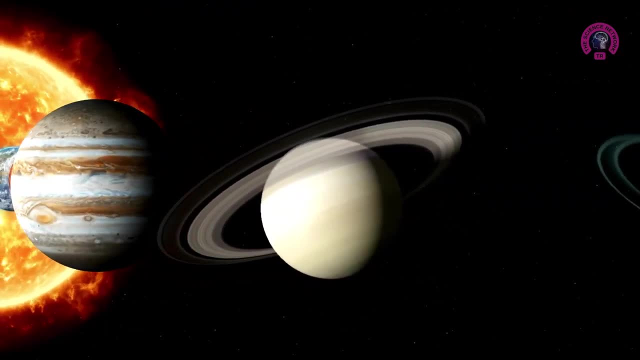 center of the universe. He was the first to discover the universe and he was the first to discover the universe. His mathematical brilliance challenged centuries of entrenched beliefs, opening the floodgates to a new cosmological paradigm that placed the sun at the heart of 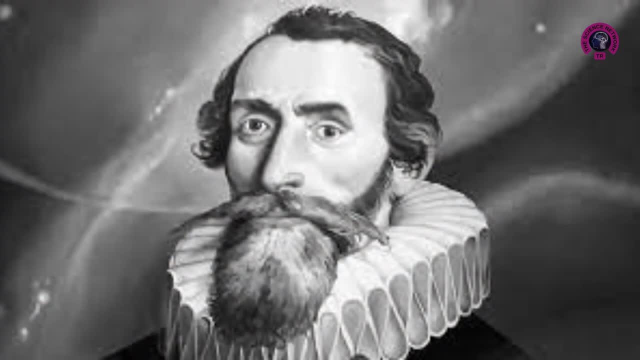 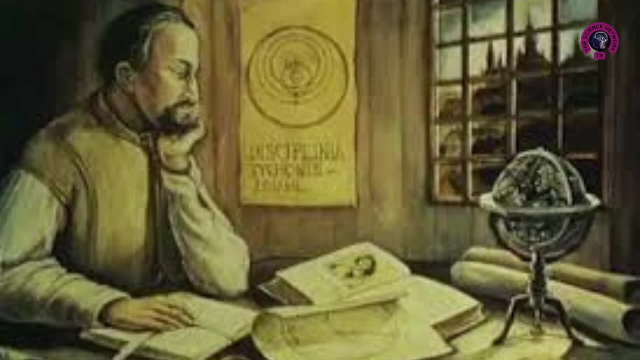 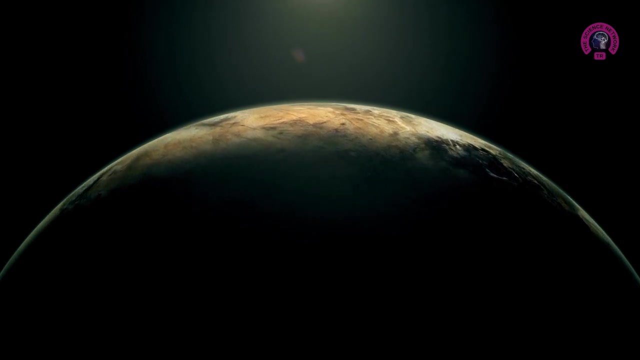 our celestial dance. The intellectual masterpiece of Johannes Kepler furthered our understanding of the cosmos as he unveiled his laws of planetary motion. Kepler's elegant mathematical formulations painted a portrait of celestial harmony, revealing the elliptical paths of planets and forever linking the motions of the heavenly bodies to the precision of mathematics. 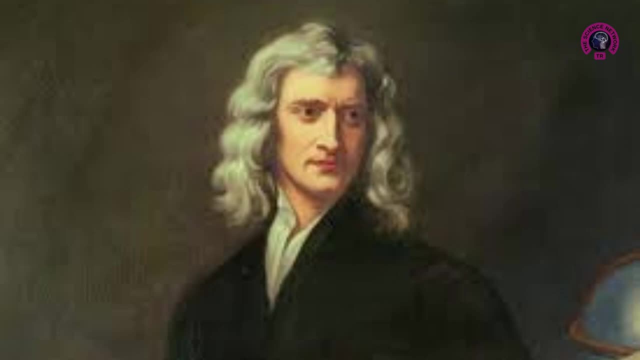 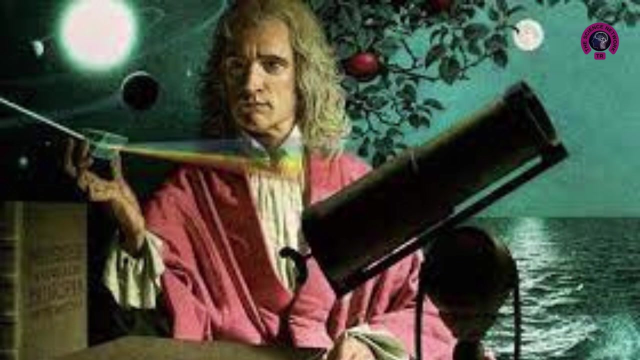 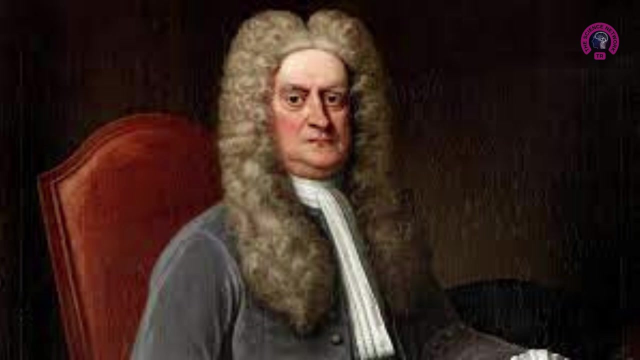 But no discussion of astrophysics would be complete without paying tribute to Sir Isaac Newton, the titan of physics. With his laws of motion and universal gravitation, Newton unified the terrestrial and celestial realms, providing a framework for comprehending the mechanics of the universe. His masterwork, Philosophiae Naturalis, Principia Mathematica, stands as a 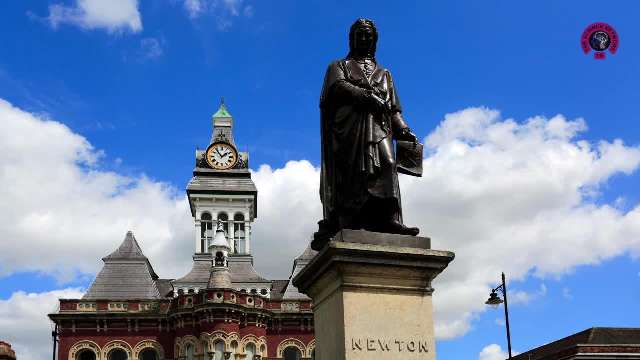 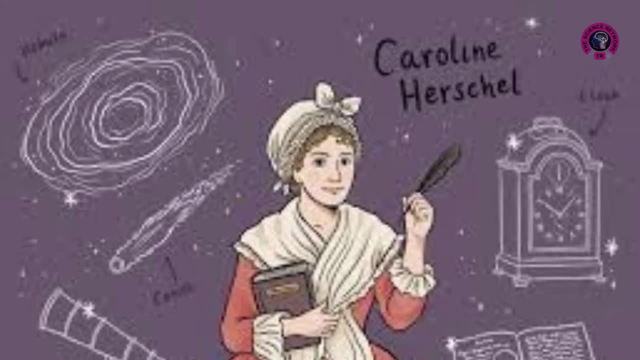 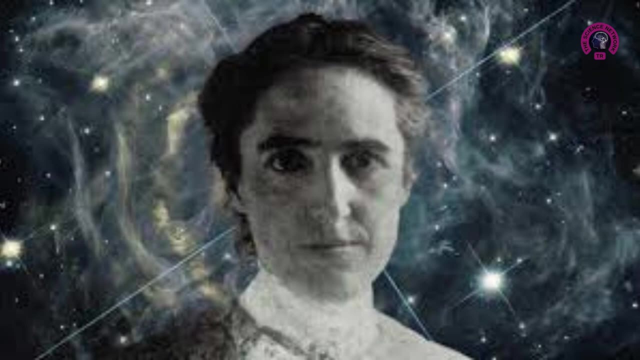 cornerstone of scientific thought, forever transforming our understanding of gravity and laying the foundation for celestial mechanics. As our journey through history unfolds, we encounter a host of remarkable minds: Caroline Herschel, whose keen eye discovered comets and nebulae, and Henrietta Swan Leavitt, whose groundbreaking work on Cepheid variable stars. 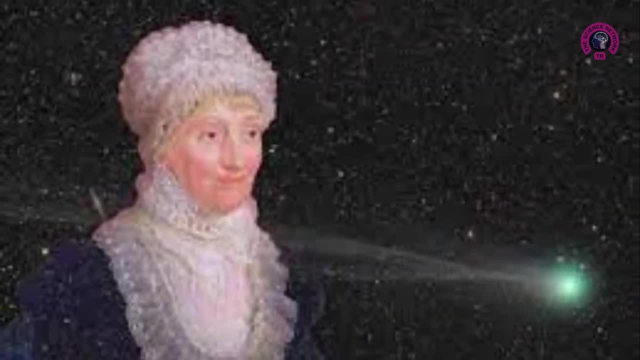 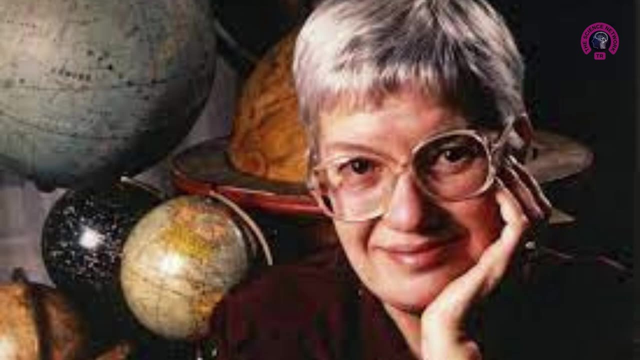 laid the groundwork for measuring cosmic distances. We also celebrate the trailblazing efforts of contemporary astrophysicists and astronomers. We also celebrate the trailblazing efforts of astrophysicists like Vera Rubin, whose groundbreaking observations of galactic rotation curves paved the way for the revolutionary concept of dark matter. 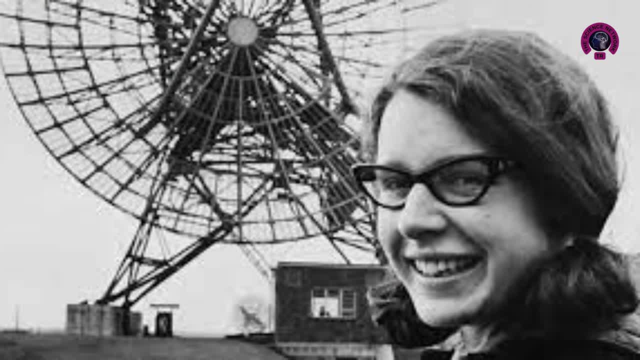 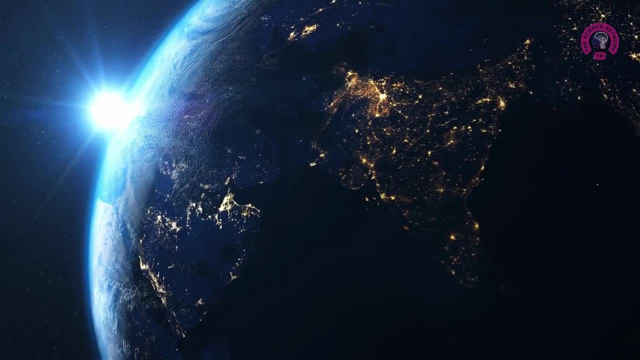 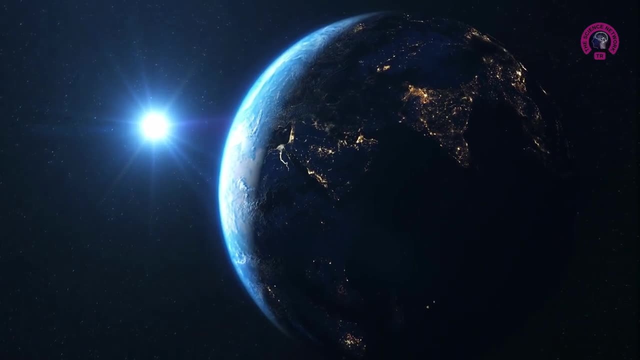 and Jocelyn Bell Burnell, who serendipitously discovered pulsars heralding a new era of high energy astrophysics. These luminaries, among many others, have sculpted the landscape of astrophysics, each adding their unique brushstroke to the grand tapestry of cosmic knowledge. Their courage,